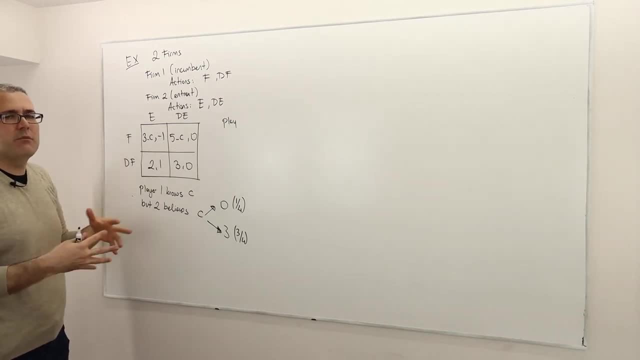 simultaneous move game, which means both players simultaneously and independently choose an action, and then the payoffs are as given: Three minus C and minus one, if firm one fights and firm two enters, for example. Well, here C is the parameter which is payoff relevant parameter, So the payoffs are private. 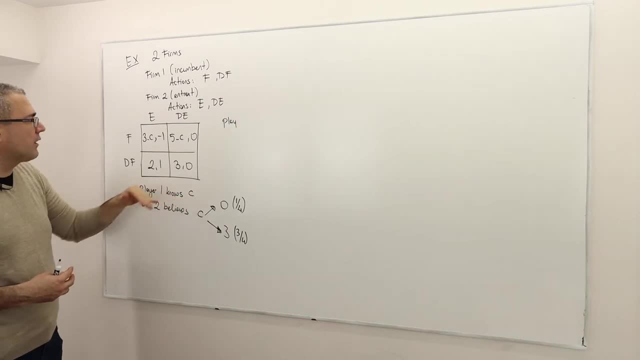 information. So player one knows the C, all right. However, player two believes that C is either zero or three. with those probabilities, okay. So if you look at this game, player two's payoff and the firm two's payoff is certain, all right. There's no type of player two, because his payoff 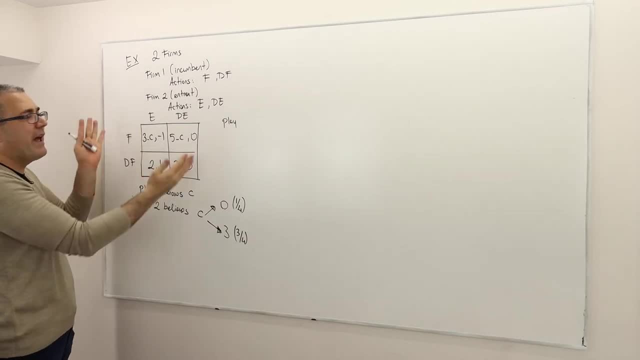 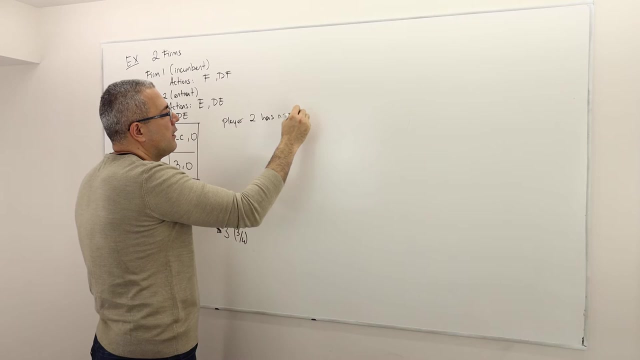 is either minus one or zero, or one or zero, depending on the strategy profile. There's no type for player two. However, for player one, there are two types. all right, So let's write it: Player two has no type. Why? Well, because the player two's payoffs are, you know. 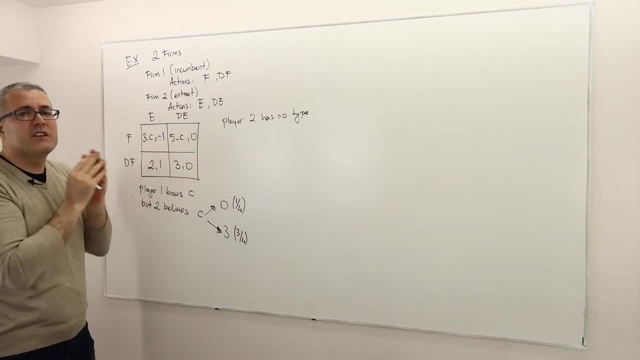 by the way, don't forget, we assume that this box is common knowledge. all right, And all this information is also common knowledge. So there's only one thing which is asymmetric: that the value of C, the true value of C, is only known to player one. all right, Player one receives this information. 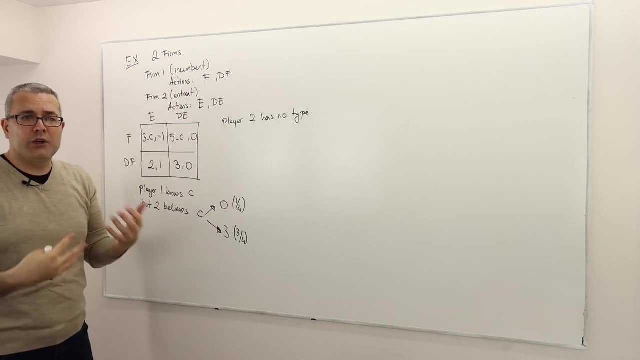 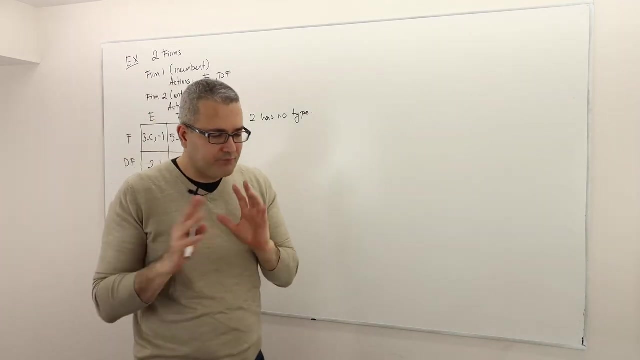 I know my C, but player two is unsure about the value of C and he believes that it is zero or three. with those probabilities, The player one knows what player two believes, all right, But player two cannot. so I mean you may wonder why. 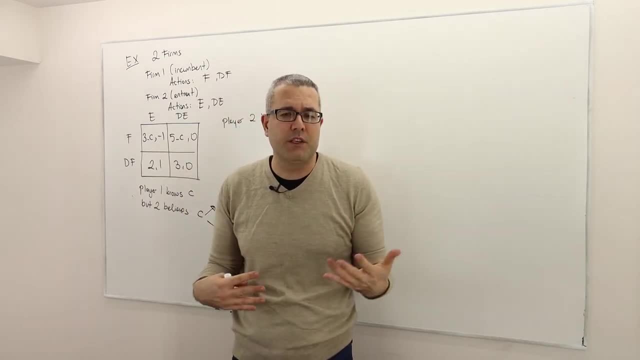 these two guys are not communicating with each other. Maybe player two is going to say: look, I am type zero or type three. Well, this type of communication is actually another strategic environment that we are not analyzing here. all right, So there's no communication between these. 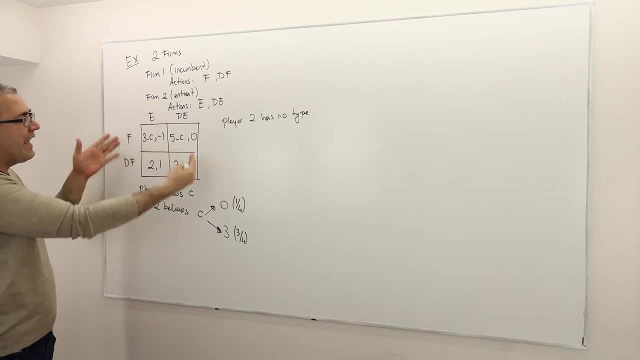 players. It's very important, All right. So this game is known by all players, which means player one is sure about player two's payoffs And, as I said, it's either minus one or zero, or one or zero, depending on the strategy profile, And so 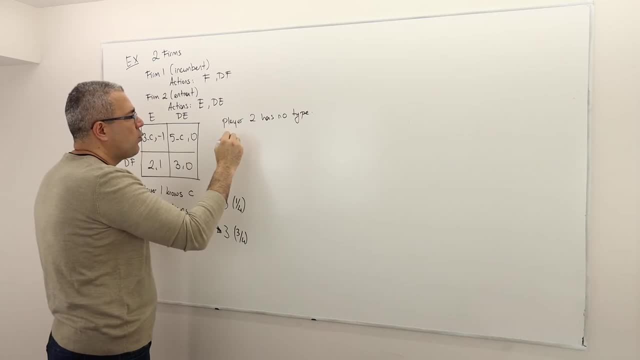 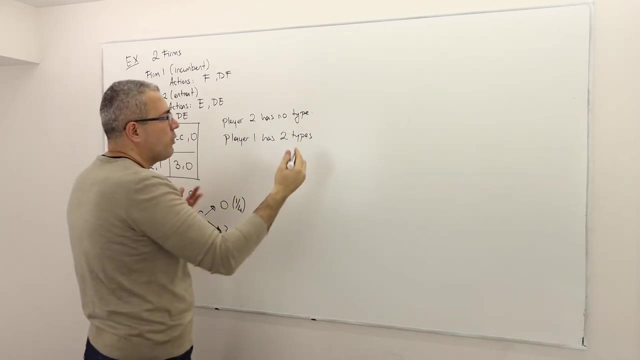 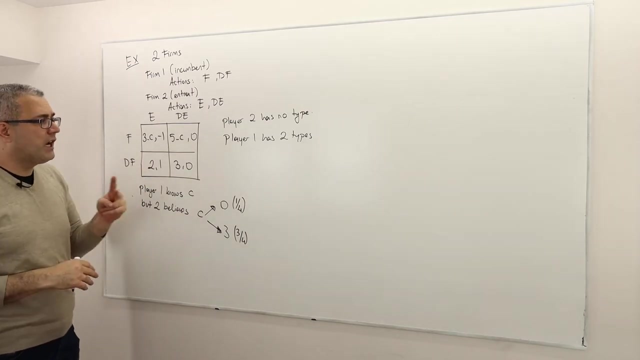 player two has no type. However, player one has two types. How am I going to denote it? I'm going to denote it by. you know, I'm not, let me skip that. Well, player one has two types, That's. 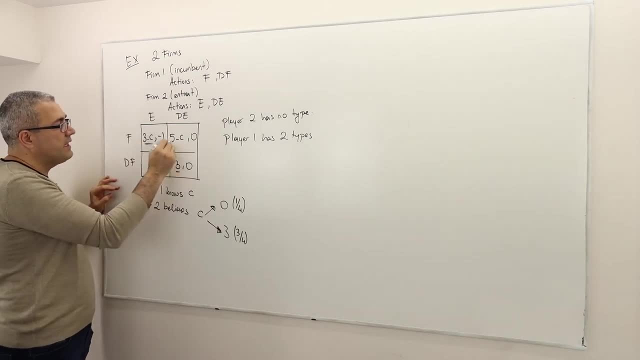 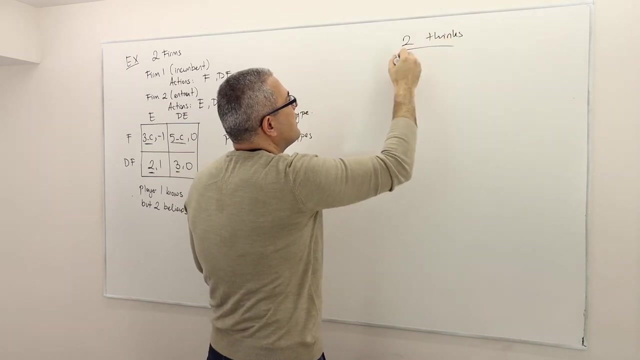 because, look, C, which is the uncertain parameter, affects only player one's payoff. All right, So because the value of C only known by player one, player two thinks that, okay, this is the. so this is what player two thinks. Two things, The game is: either C equals zero, 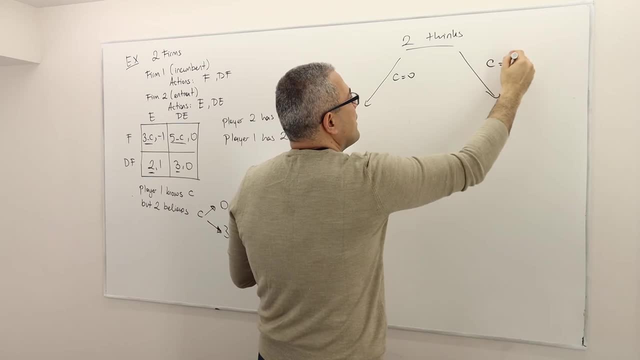 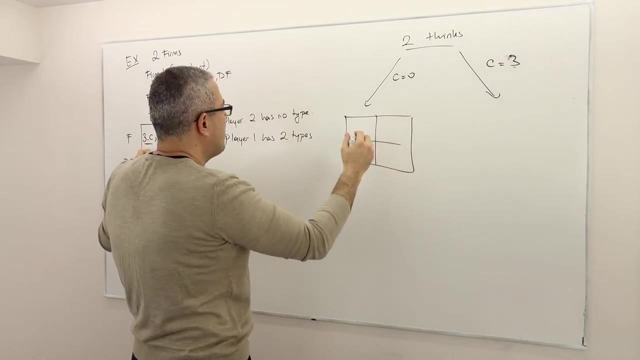 or it's, I'm sorry, not four. C equals three. Well, in this case, if C is equal to zero, well then the game is in fact three minus zero and five minus zero. All right, So it is this. 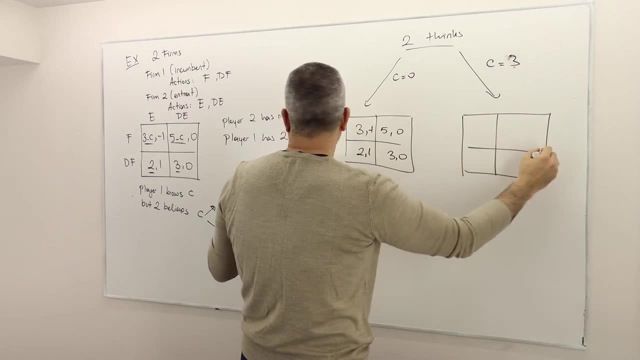 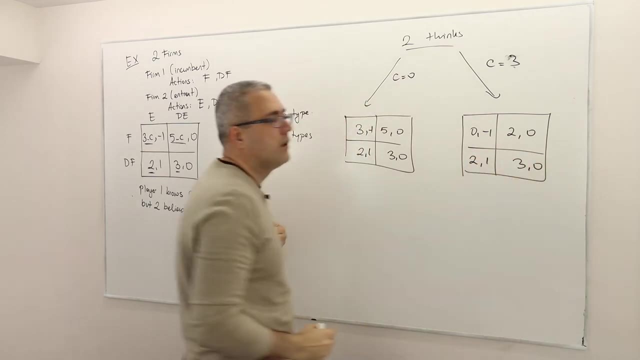 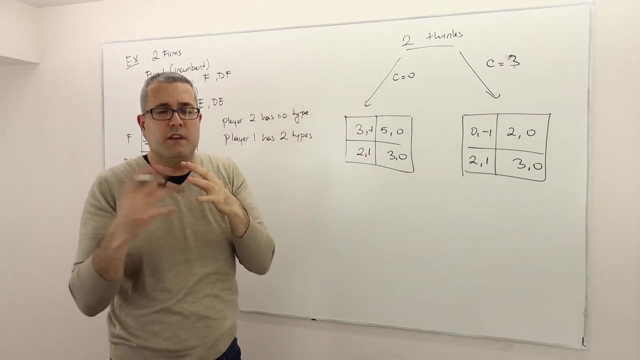 And if C is equal to three, well then the game is zero minus one. two zero two. one three zero. Okay, So the the player two things. he is playing a game with his opponent. player one: right. This is player two. 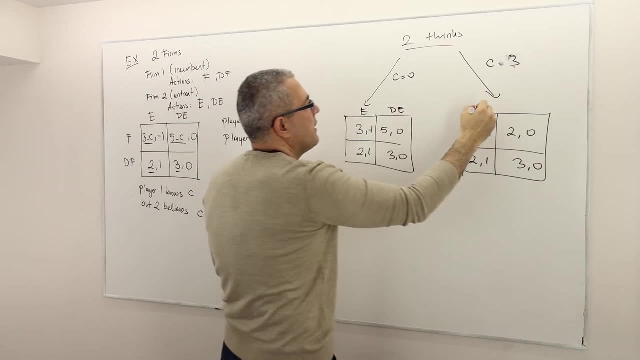 So he's going to choose E or don't E, E or don't E. But the thing is, his opponent is going to fight or don't fight, fight or don't fight. So once, for example, his opponent chooses fight and player, 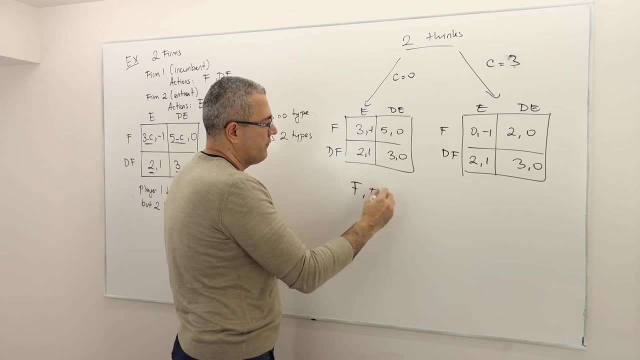 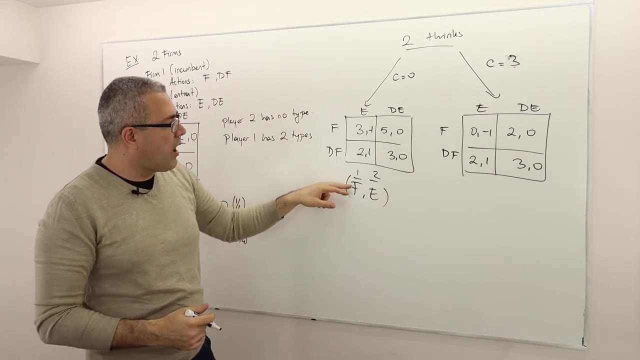 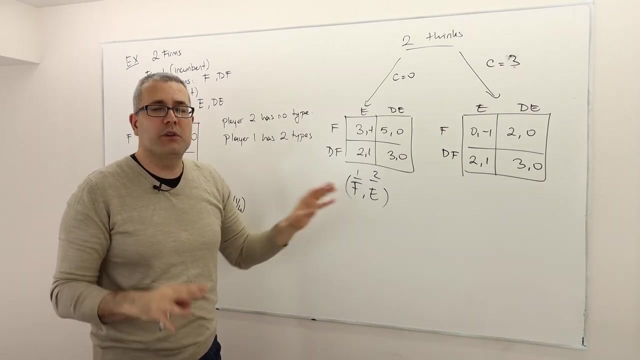 two things: enter right, Fight enter, for example. So this is what player one plays, This is what player two plays. So here player one will know about his payoff. All right, Again, assuming that player one plays fight, player two plays enter, and this is common knowledge for 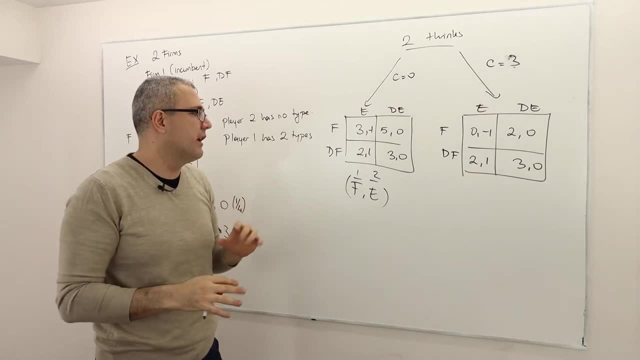 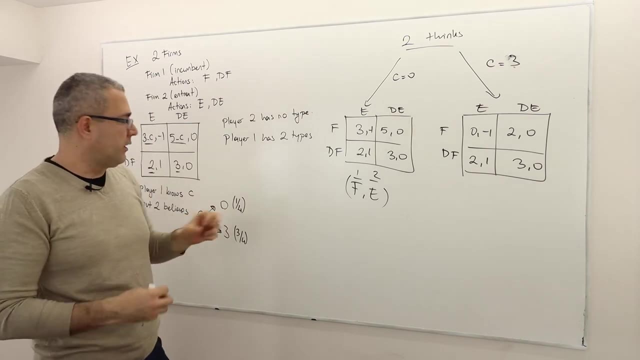 some reason- let's suppose this is known- before they played the game. This is a hypothetical situation. Player one is going to know his payoff. Well, if C is- sorry- zero, he knows that his payoff is going to be three. If, however, C is three, he will know that his payoff is going to be three. 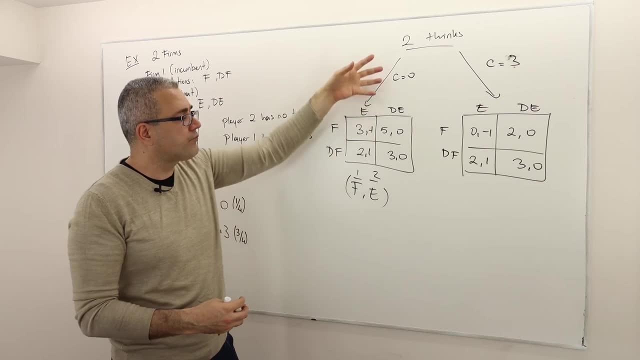 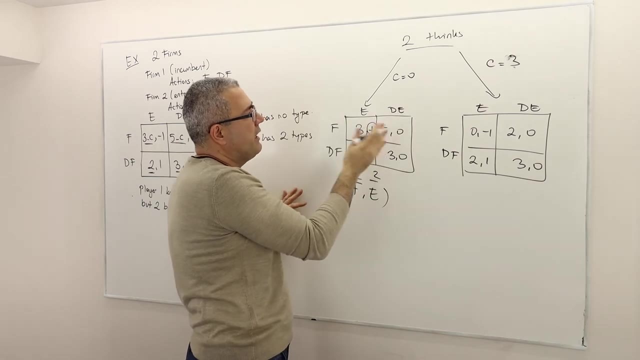 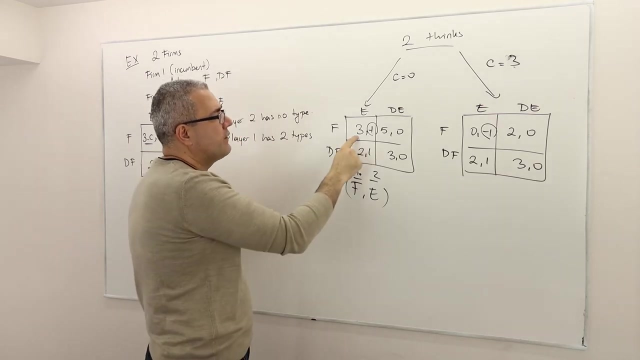 He will know that his payoff is zero. However, player two is unsure about this. Well, is my opponent meaning am I going to get? well, I mean, in either case, he's going to get minus one, All right. However, he is unsure about his opponent's payoff, right? So it could be this. 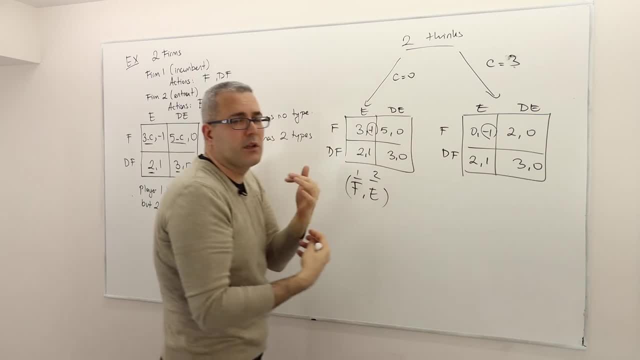 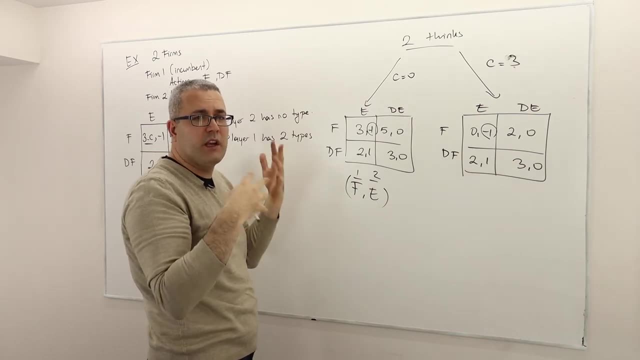 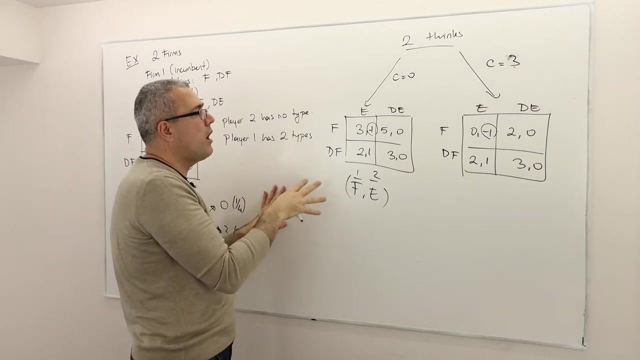 game that they're playing, or it could be this game that they're playing. So, once again, player two's payoff is fixed in either game. However, if C is sorry- zero, he knows that his payoff is. However, that's not why we generate two types for player one. We generate two types of player one. 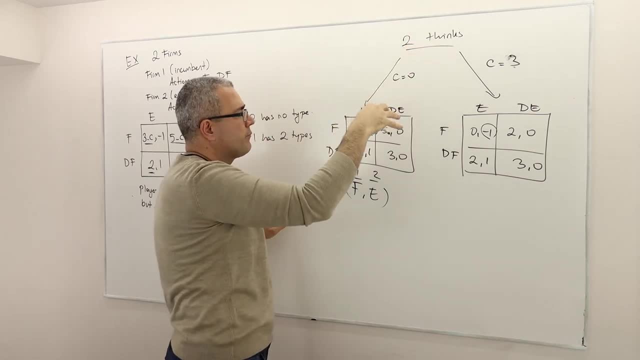 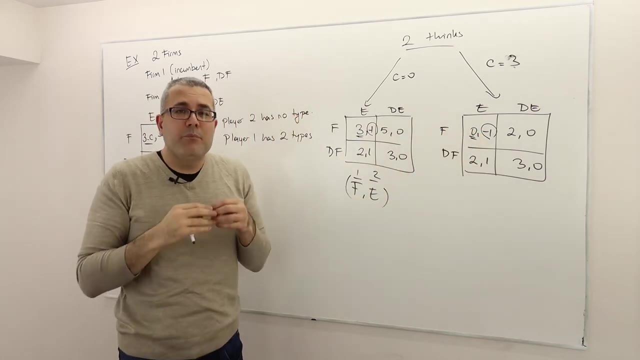 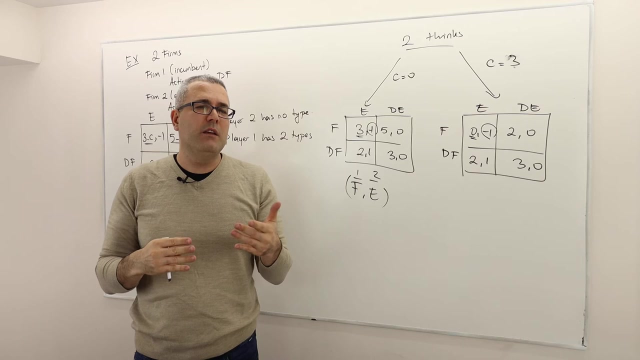 because player two is unsure whether player one is going to get three or zero. Well, why does that matter? Well, because if you are unsure about your opponent's motivation, you cannot really be sure about his best response or his optimal strategy. So therefore, you have to calculate your best response by taking an. 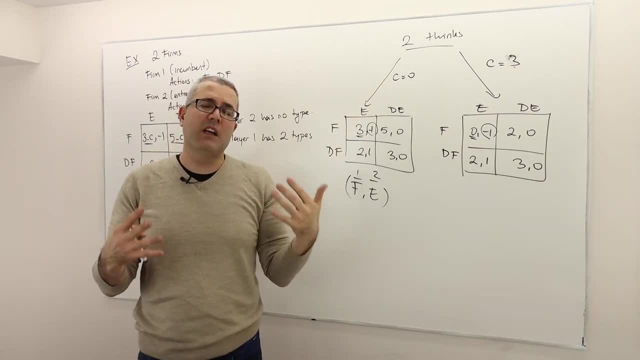 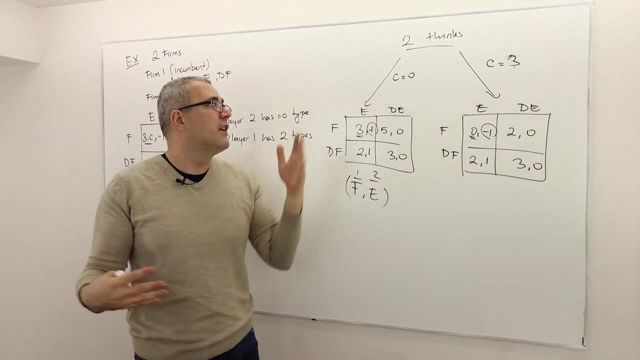 expectation. So, therefore, player two is the guy who's going to take expectation in this game. Well, expectation of what? Well, the game can be either this or that. What does that mean? That means your opponent can behave one way or another way, depending on the value of C. So therefore, 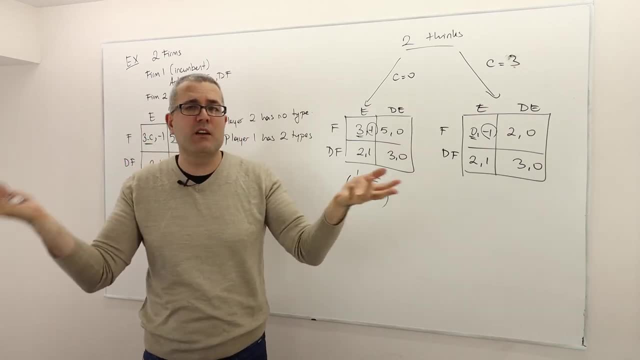 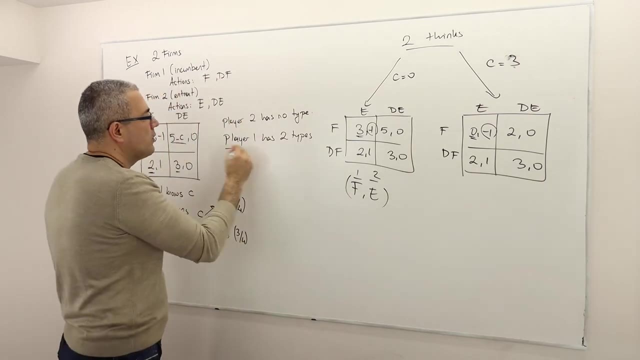 your opponent. player one can behave either one of these two ways means the player one has two types, right, Not player one. So player one has two types. That's that's very important And I hope that is clear because you. 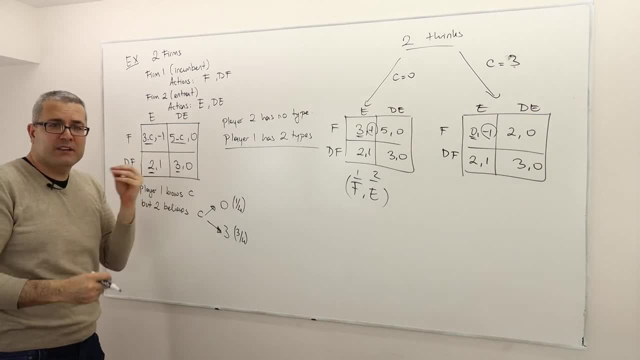 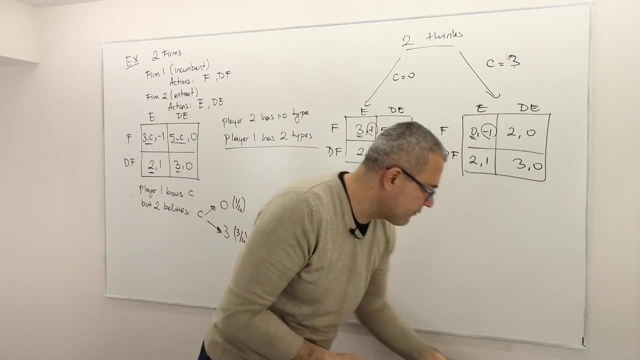 have to be clear about which player has how many types and what types belongs to what player. So that's that's an important part of analyzing this, this, this type of game. So the question is asking us to find the Bayesian Nash equilibrium. 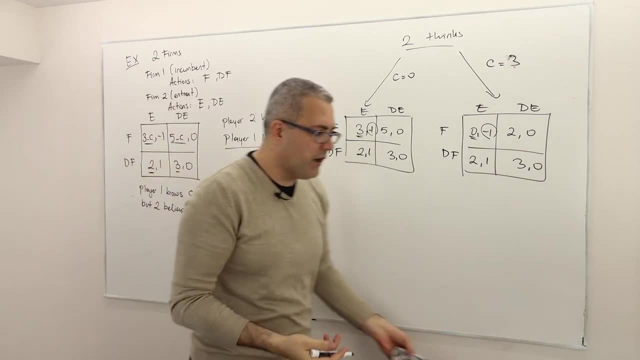 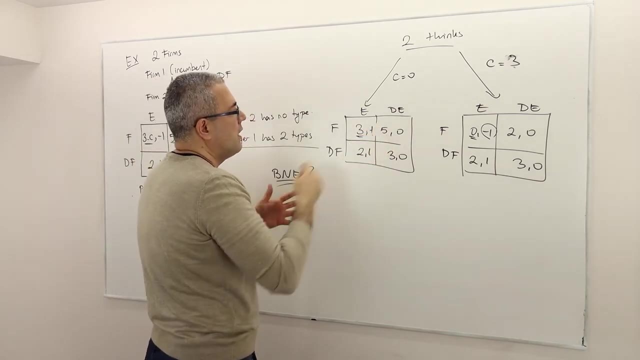 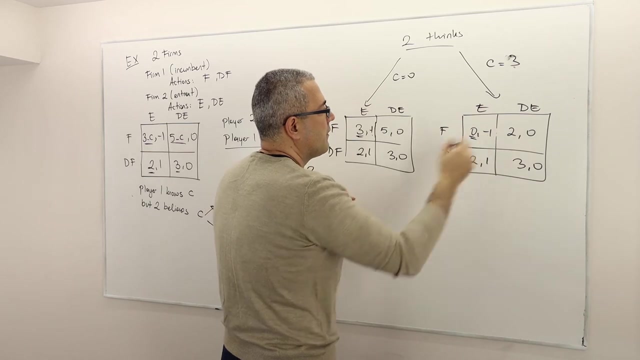 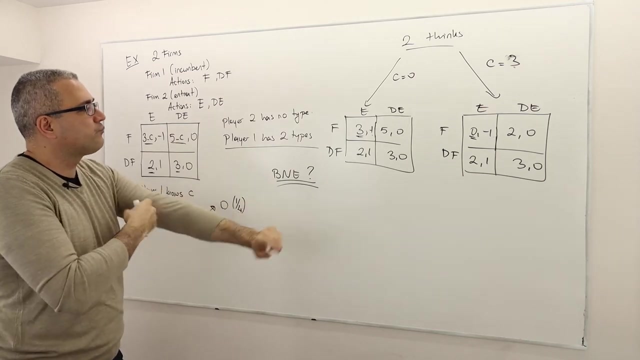 equilibrium of this game. is there any? is there one? is there multiple? Okay, So how are we going to do that? Well, you can check and verify, Right, But obviously, what I'm going to do is the following. So let me take this into account. Alright, so here is the player ones. So here, Player one. 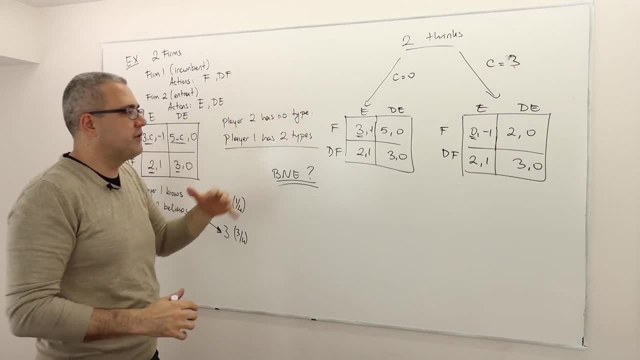 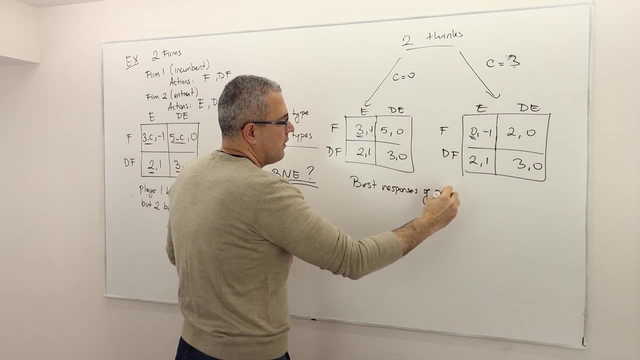 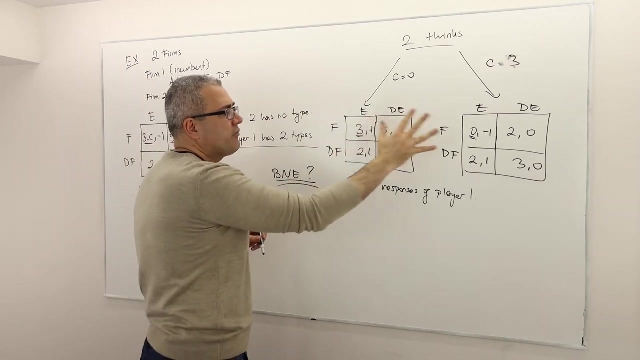 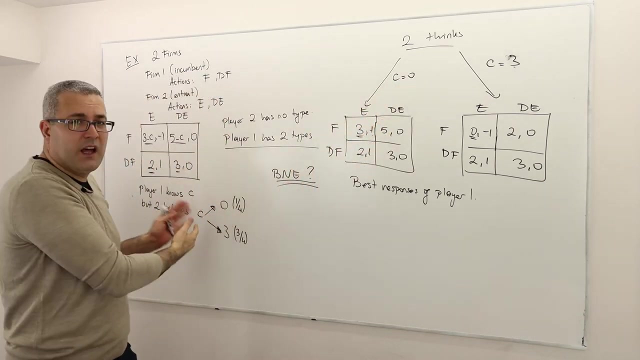 let's look at the player one's optimal strategies. All right, best responses. Best responses of player one: Well, if player two? well, remember, player one knows exactly what metrics he is playing. So, if C is equal to zero, he knows the value of C, but we, as the analyzer, do not know it. So therefore, 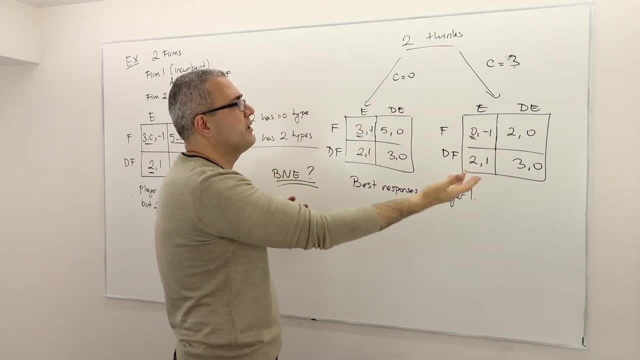 I need to check his optimal strategy in each case. So if C is zero player, one is going to know that this is the game. If this is the game, what is his best response? Well, if his opponent player two plays E enter, well, his best response is clearly fight, because three is higher payoff than two. 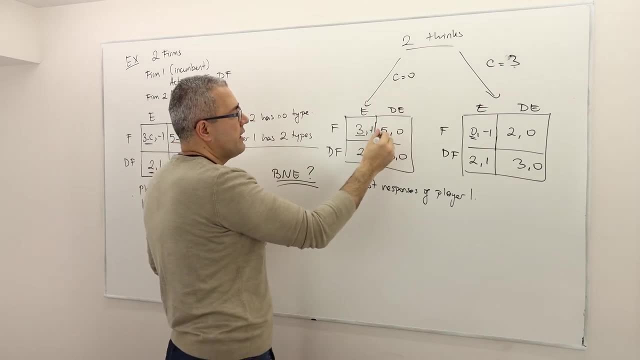 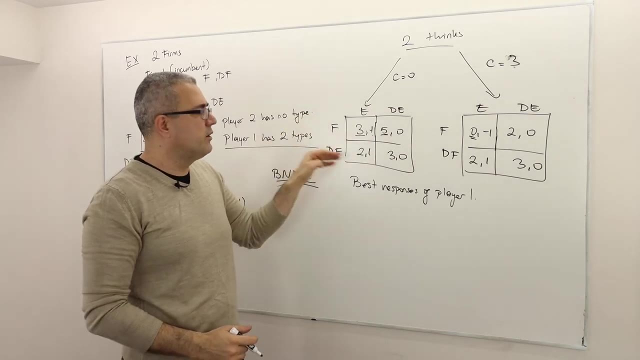 If his opponent doesn't enter, his best response is: again fight. Well, if you look those payoffs carefully, you will see that C is zero. So if C is zero, player one is going to know that this is the game. So carefully: fight is strictly dominating, don't fight, All right. so what does? 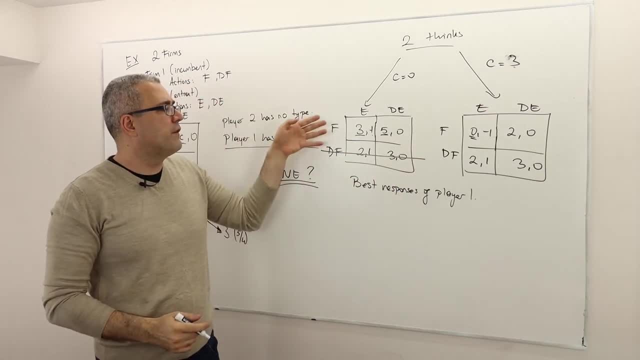 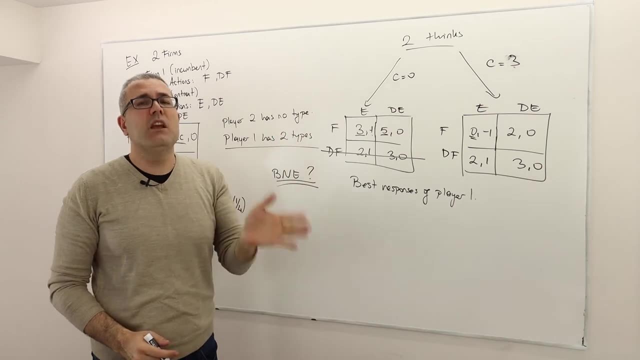 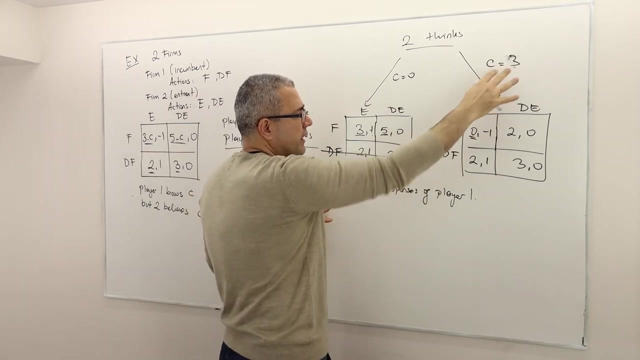 that mean. That means player one will never play. don't fight. in this case, If C is equal to zero, then fight is the only strategy. That's very good. Well, what about here? Well, here, if C is three, player one is again going to know that this is the metrics And what is his best. 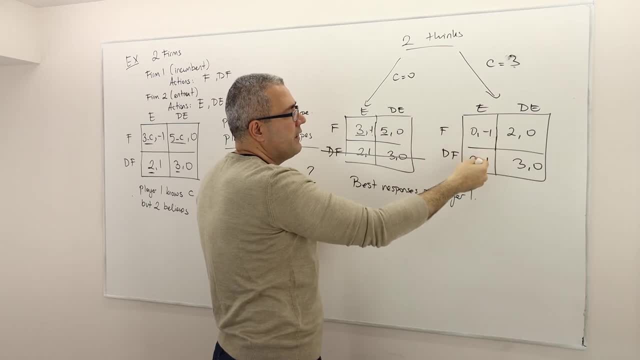 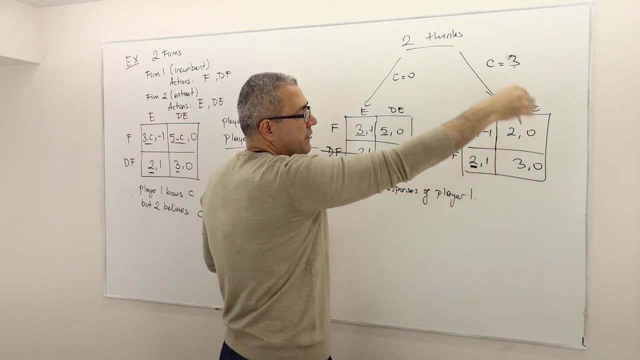 response. Well, if his opponent enters, he has the best response. So if C is three player, one is he is going to prefer to don't fight because two is a higher payoff than zero. However, if he enters, if his opponent doesn't enter, 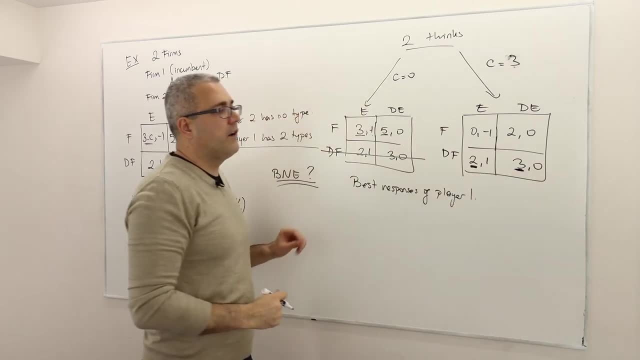 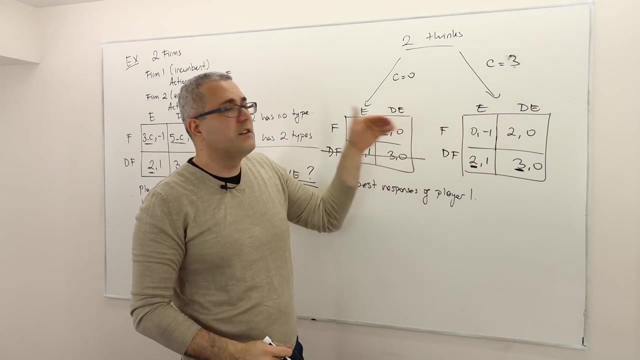 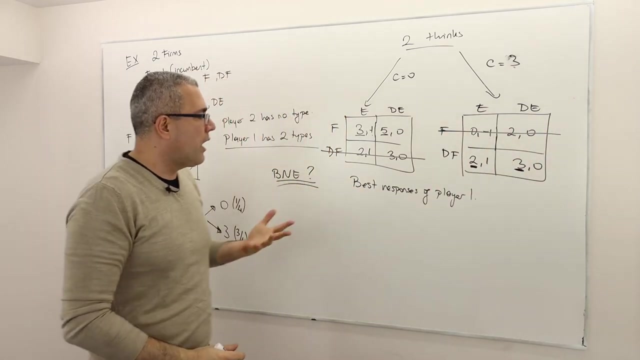 well, this time again, doesn't fight is an optimal strategy. So, once again, if you look at those payoffs, don't fight is strictly dominant strategy, meaning it strictly dominates fight. So what do I learn? We learn the following: 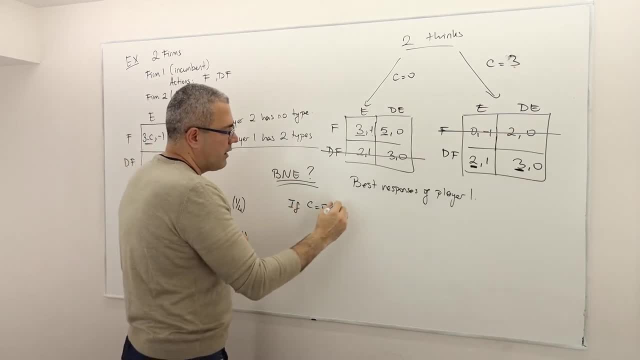 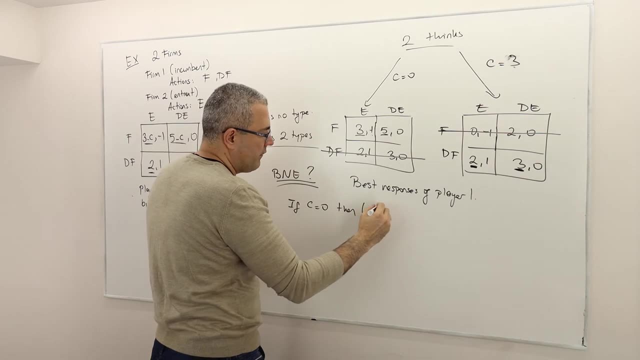 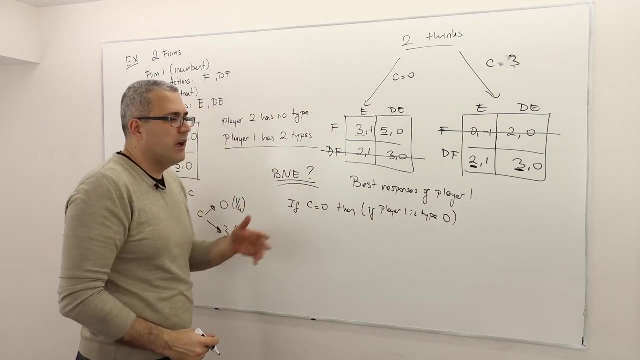 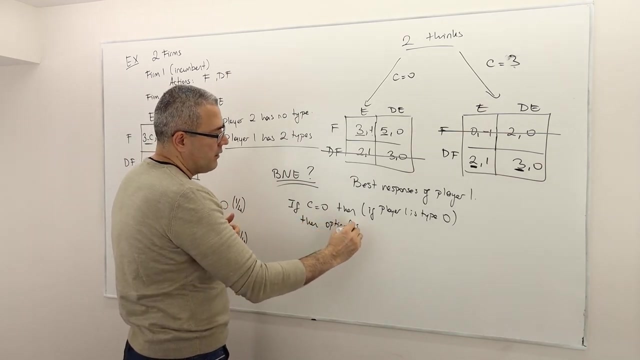 If C is equal to zero, then meaning if player one is of type C equals zero. you can think it that way. If player one is type zero, OK, I just named this case and I call it type zero case. Well then, optimal strategy, because it is strictly dominant strategy. 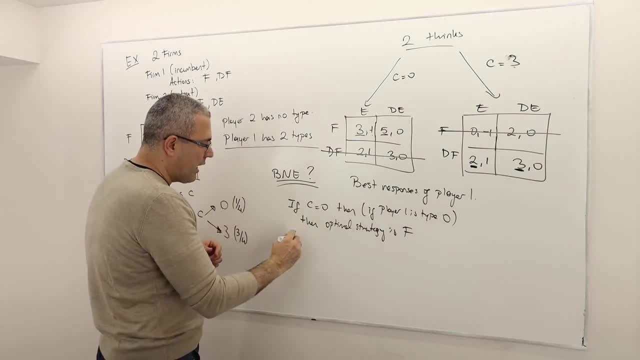 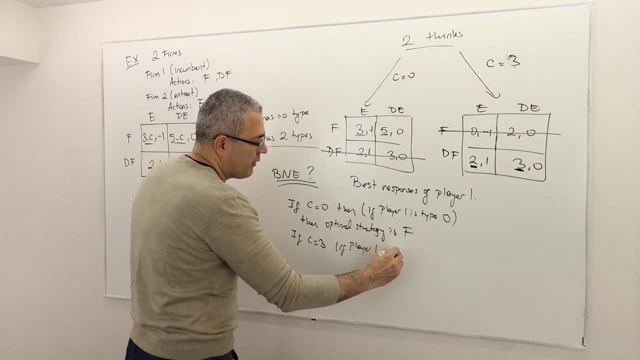 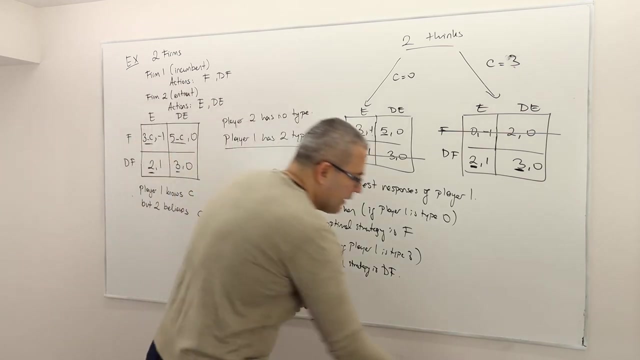 strategy Is fight, And if C is equal to three, or if player one is type three, well then, optimal strategy is: don't fight, All right. So what does that mean? That means, if I am looking for Nash equilibrium, let me erase these. 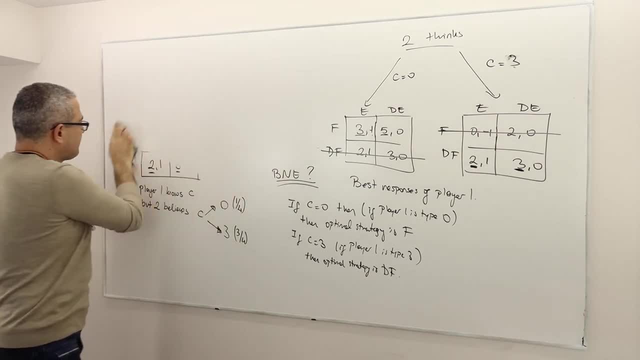 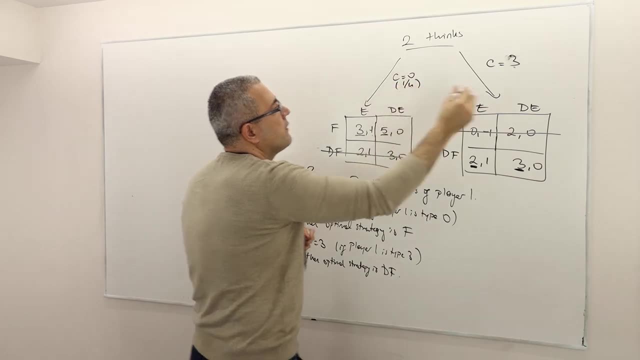 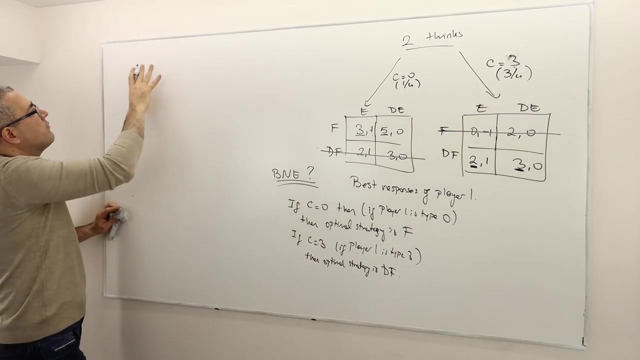 because I need some space. Here is what I have. Oh, one, fourth, three, fourth, Don't forget, this is one over four, This is three over four probabilities. So this is what I have. I already found. So, remember, you have to be clear about what strategy profile will look like. 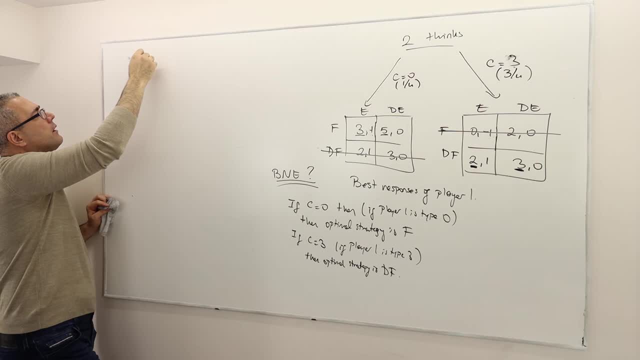 So there's two players, player one and player two. So, remember, player one has two types, So his strategy is going to be player one strategy, Player one, strategy of type zero and of type three. All right, So this is how I'm going to denote them. 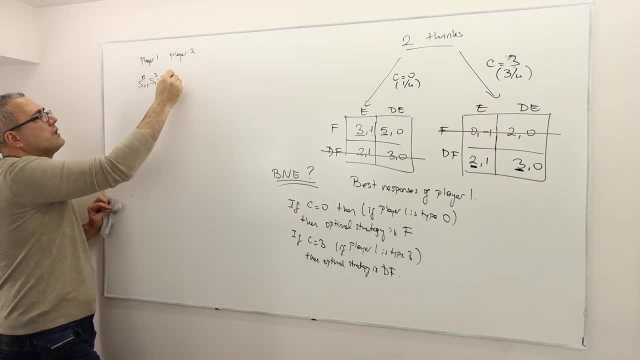 All right. And then player two strategy is going to be S2.. So this is what a strategy profile, or Nash equilibrium- Bayesian Nash equilibrium strategy profile- will look like. So there's going to be three components, because there are two types of player. one: 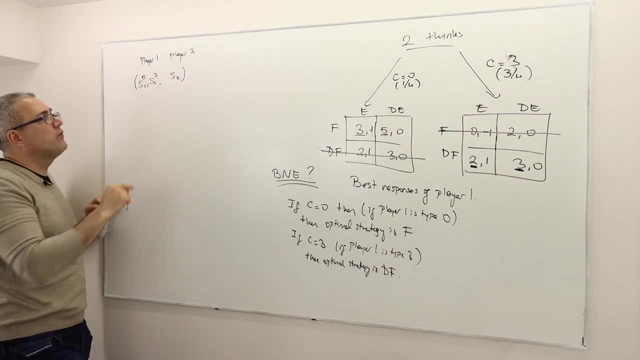 And one type of player two. We already found the best response of player one of either type. If it is type zero, well then, he's going to play fight. If it is type three, well, we already know that it is going to play, don't fight. 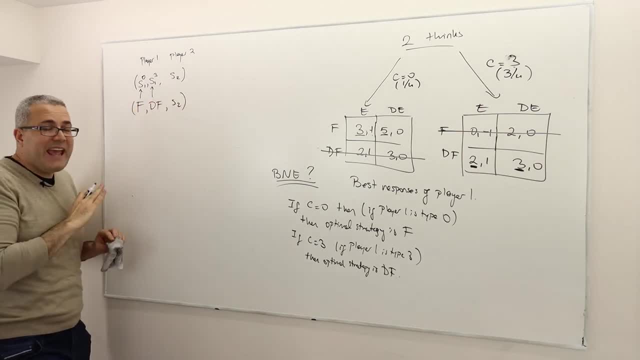 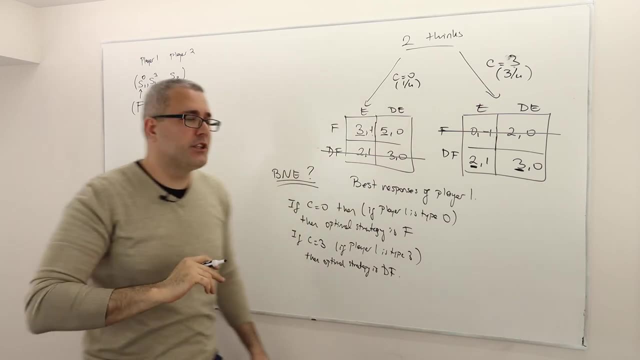 So fight, don't fight is the strategy in any Bayesian Nash equilibrium. These are the strategies for player one, All right Again, in any Bayesian Nash equilibrium. The question is, maybe we have more than one Bayesian Nash equilibrium. That I don't know yet. 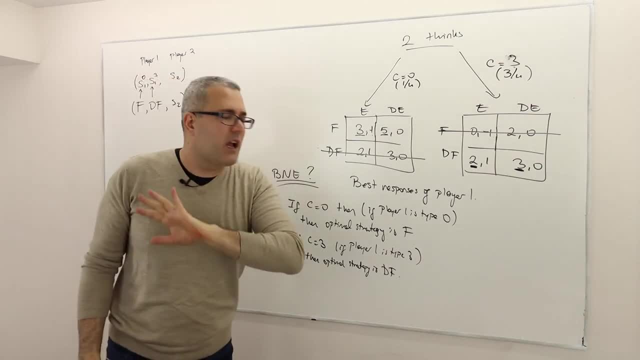 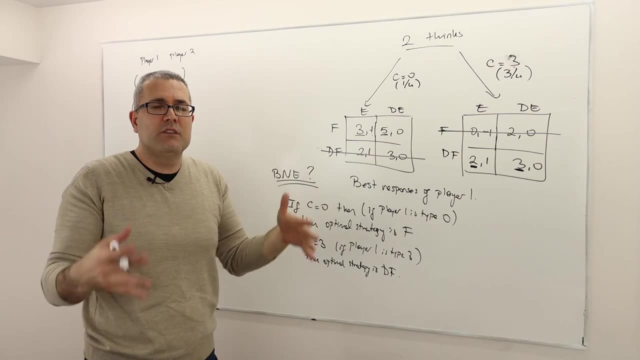 But what's going to be S2?? A big, a common, huge mistake is I mean in this game. sorry, both approaches may lead to the same outcome. I don't know it yet, But you can say: player one, I'm sorry, player two. 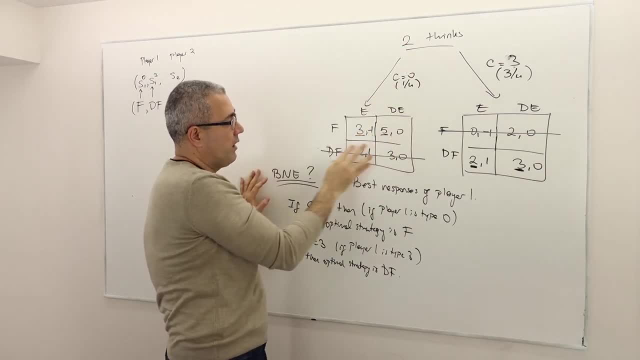 If this is the game, clearly this is mine. Well, we know that player one is not going to play- don't fight, right? So therefore, he knows that fight is what player one is going to play, In which case it's going to prefer to play. don't enter. 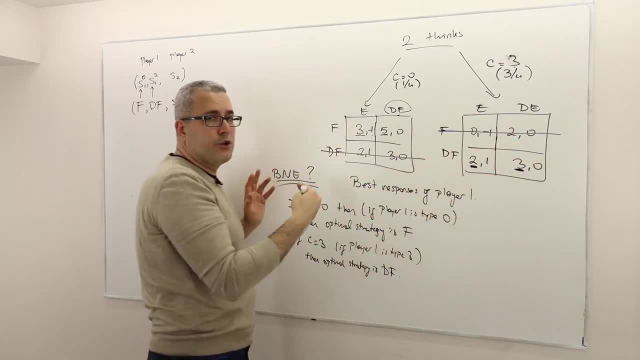 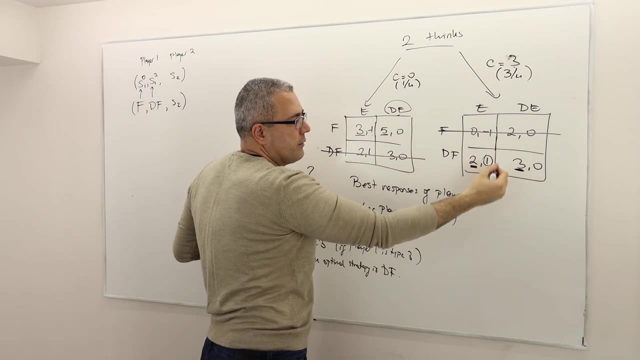 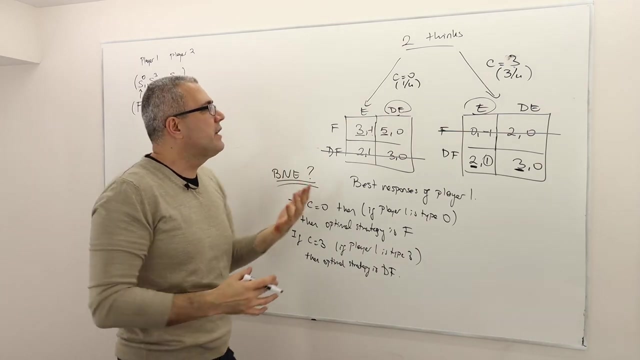 And in this case player two knows that player one is not going to play fight. So therefore for player two, enter is the best response, Because the payoff is one rather than zero. So he's going to play enter here. But the problem is, you cannot say two plays. 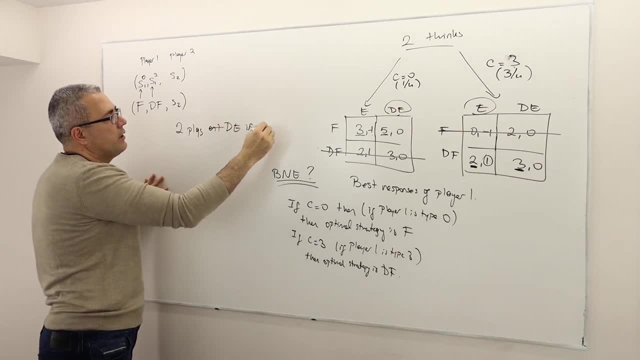 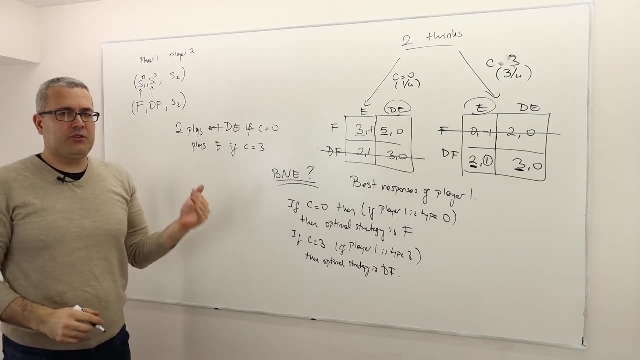 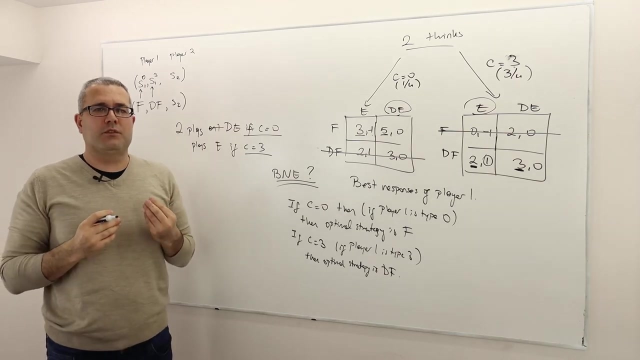 Sorry, don't enter If C equals zero And two plays enter if C equals three. This is not a strategy. Why not? Well, this, if condition player two will never observe C equals zero, And so you cannot expect him to condition his strategy with overseas? 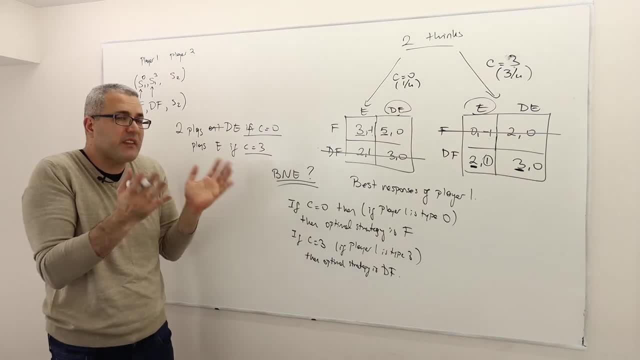 Like I can't. I mean he can't play. if C is zero, I'm going to do this. If C is three, I'm going to do that. But what if you don't know? You don't know what C is. 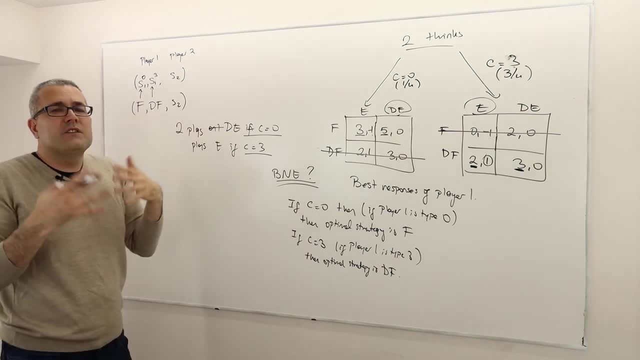 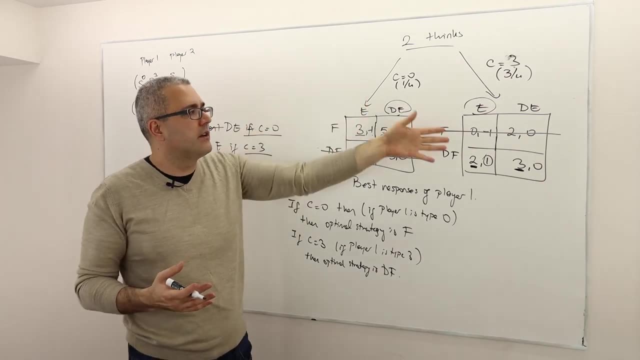 What the heck are you going to do? Well, so player two is supposed to choose just one action: enter or don't enter. But which one One is better sometimes, The other is better other times. So for that reason you have to take the expectation. 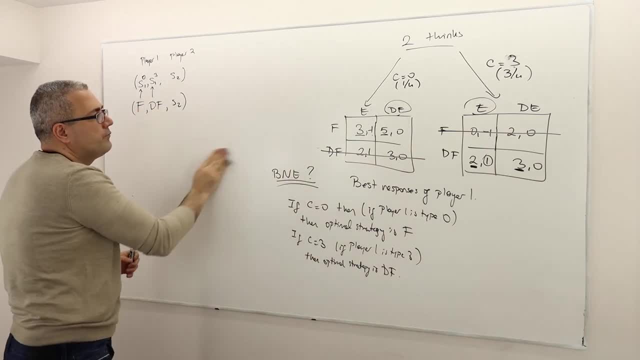 So how do we find the best response for player two? Well, this is what he's going to do. Well, what is the expected utility of player two? Given that player one right, We can fix player one's strategy. FDF. 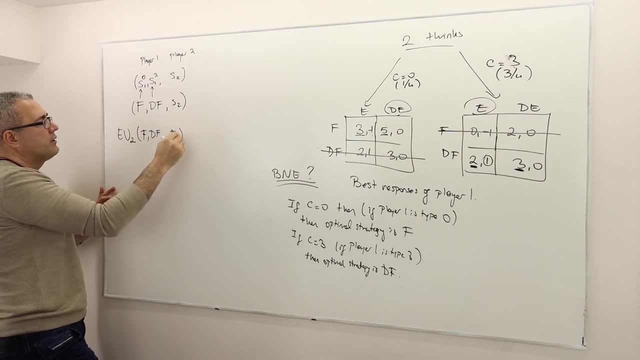 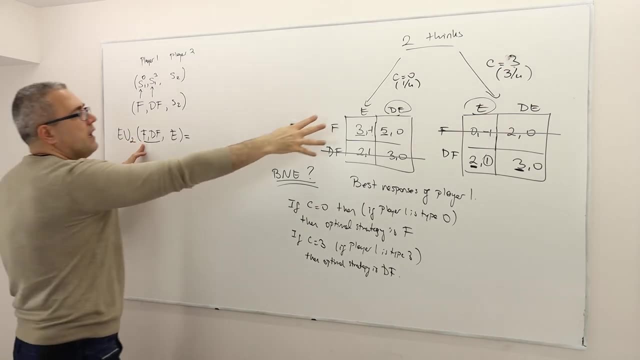 All right, And player two plays enter. So what is his expected payoff If he plays enter, given that player one plays F? if he is this type and doesn't don't fight if he is this type? We fixed already those because we know that these are optimal strategies in any Bayesian-Nash equilibrium. 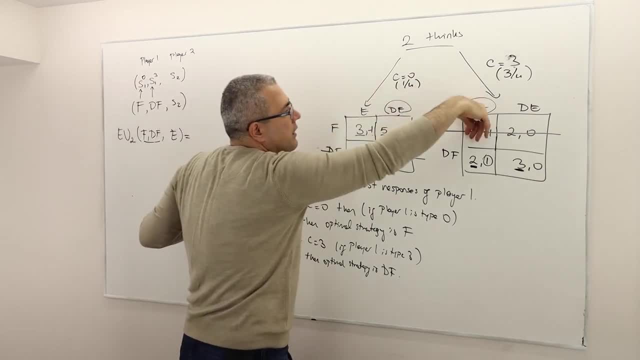 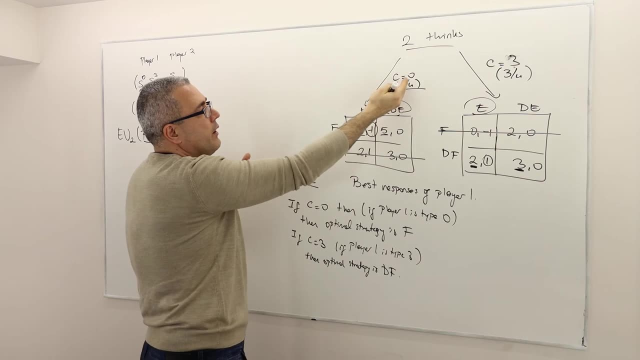 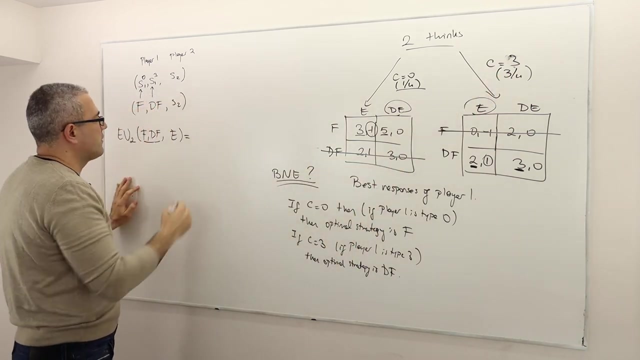 Well, so that means if he chooses enter, he's going to get minus one payoff, with probability one over four, because he's going to get minus one payoff if C is equal to zero, And he's going to get again minus one if C is equal to three. 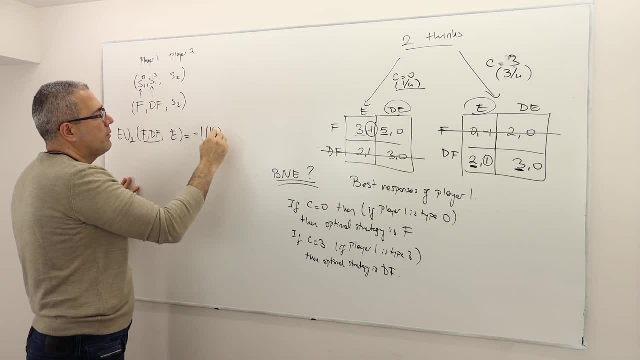 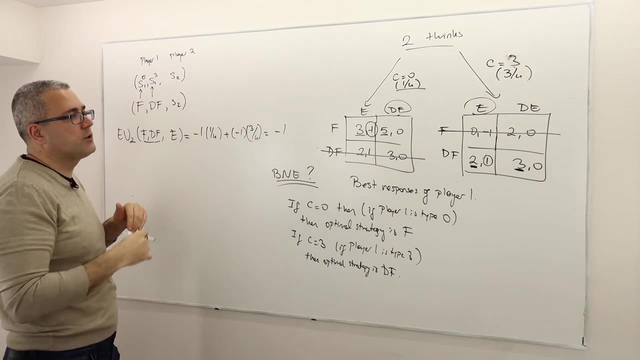 So he's going to get minus one with one over four probability, plus minus one with three over four probability, So it's basically minus one. All right, He's going to get minus one anyway. So I am so sorry, Yep, That's my mistake. 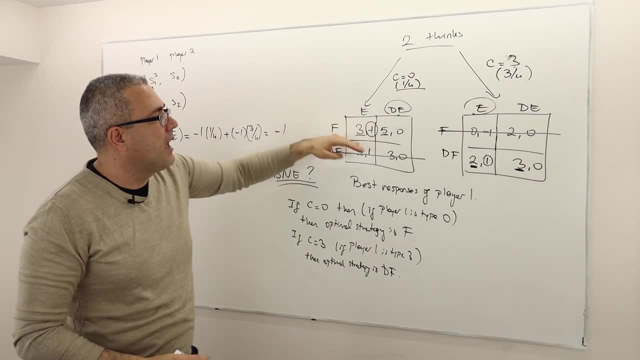 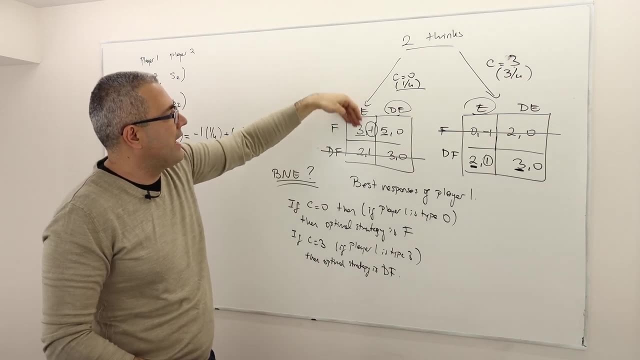 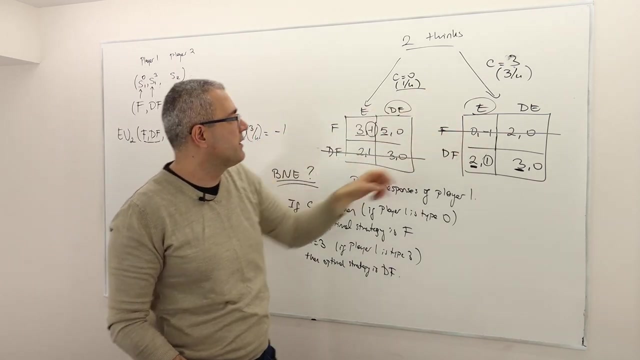 So remember, player one is playing fight here and don't fight here. So yeah, be very, very careful. So here, if player two plays enter, he's going to get minus one because player one is playing fight. But here he's not going to get minus one because player one of type two is not playing fight. 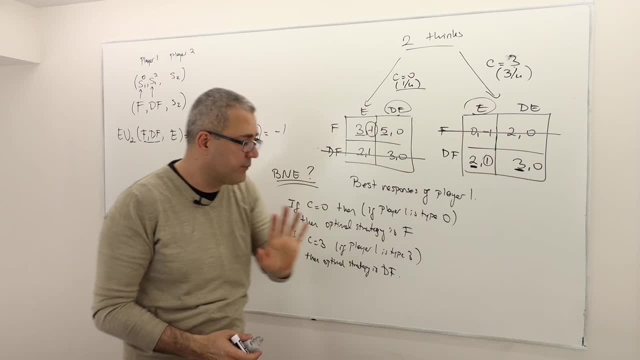 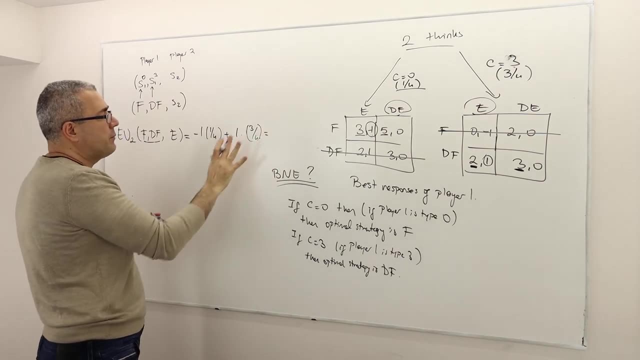 He's playing don't fight, So he's going to get one. So I am sorry That's my mistake. So this is one times three over four. So therefore the expected payoff is going to be two over four, which is equal to one over two. 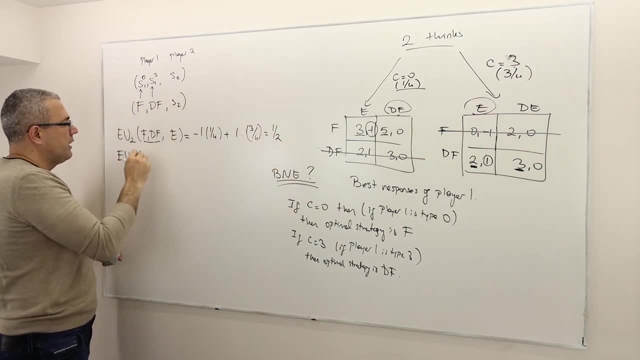 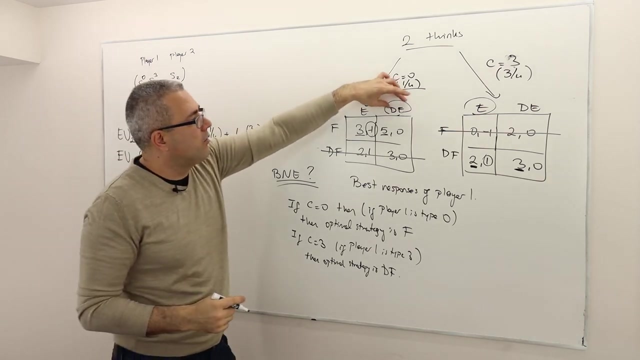 What about expected utility, Given that these are the strategies of player one? and player two plays, don't enter right? Player two has only two strategies: Enter, don't enter. Which one is optimal? Well, if he plays, don't enter in this game. 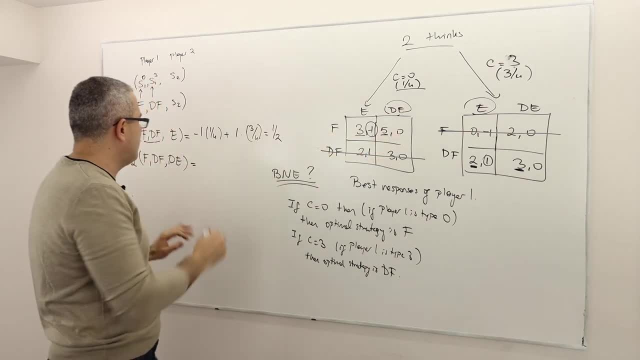 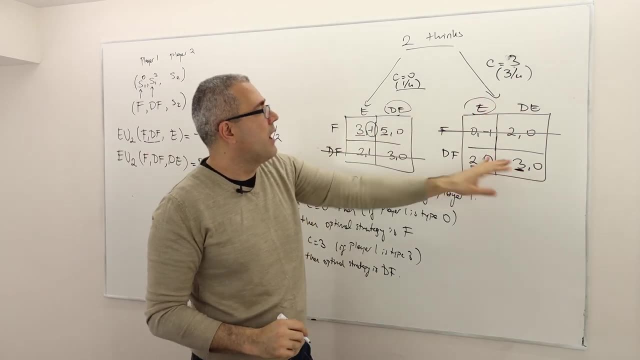 because player one is playing, fight he's going to get zero payoff. So zero times one over four probability plus If he plays, don't enter. and in this game we know that player one is going to be playing: don't fight, He's going to get zero. 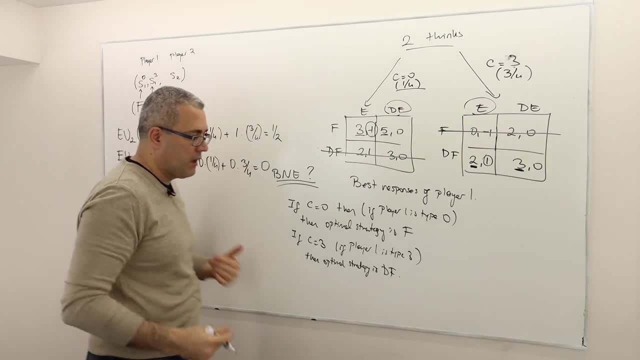 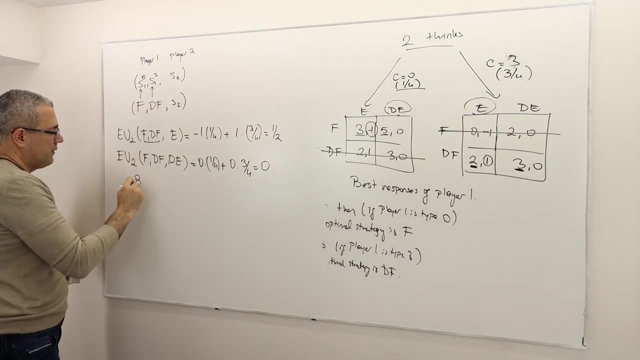 So zero times three over four, So it's zero. Very good, That's it. So what does that mean? That means because one half, Which is expected utility of fight, Don't fight E is greater than zero, which is the expected utility. 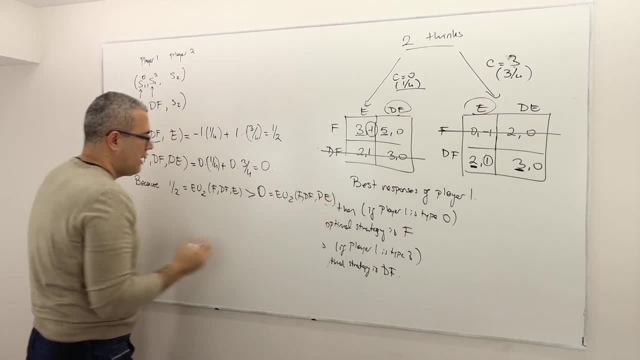 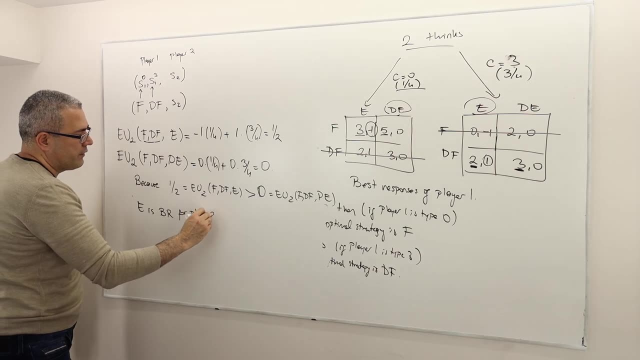 Fight, Don't fight, Don't enter. Enter is best response for player two. Hence, Look, player one of type one has a unique best response. Player two, after player one of type two, has a unique best response: DF. And we just found that player two has also a unique best response. 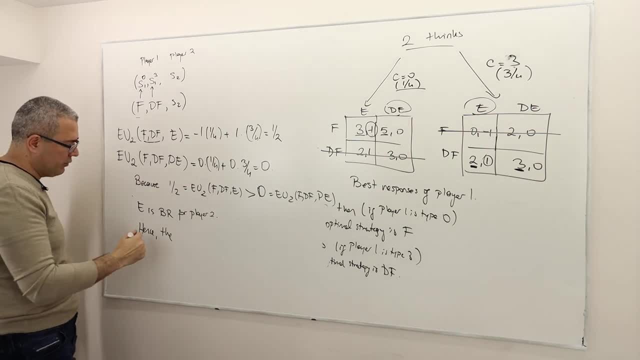 Therefore, there's going to be a unique Bayesian Nash equilibrium. Hence there is a unique meaning. There is no other Bayesian Nash equilibrium in this game. There is a unique- in pure strategies At least unique Bayesian Nash equilibrium, Which is Fight. 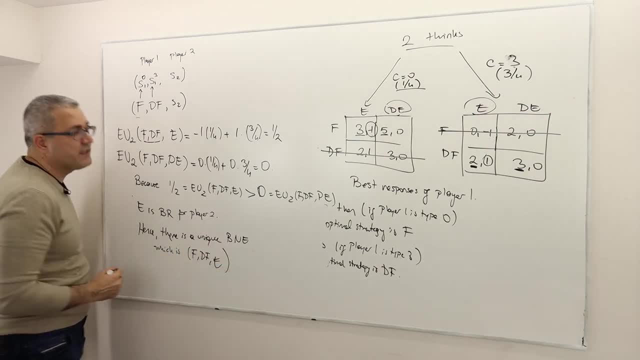 Don't fight. Enter. What does that mean? That means Player one. If C is zero, he's going to or it is going to fight. If C is three, it's going to don't fight, And player two will choose. enter. 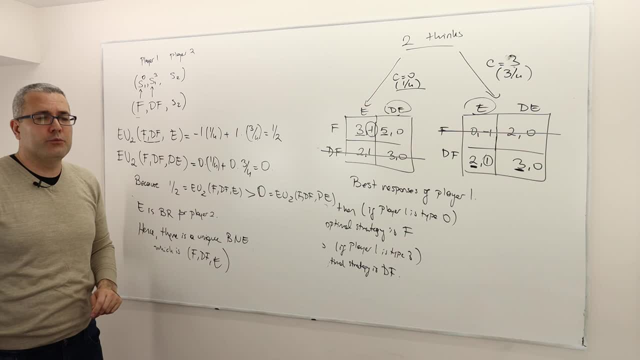 All right. So that's what the Bayesian, only Bayesian, Nash equilibrium is in this game.